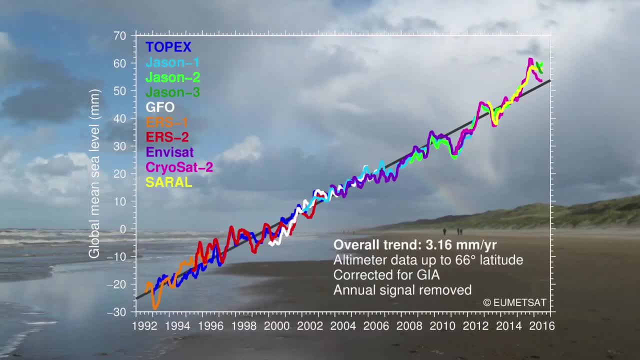 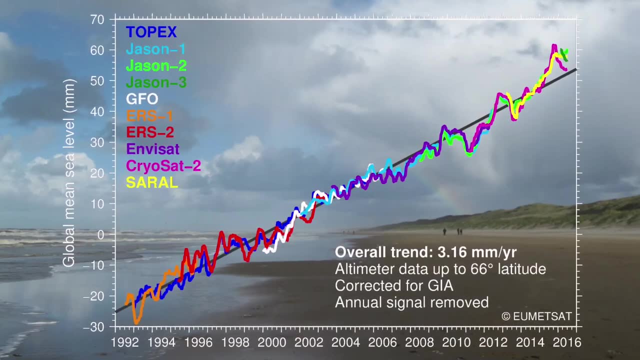 Don't forget, on top of it are tides When you normally would just survive a high tide. now you might not survive a high tide anymore, And this rise is remarkably consistent, isn't it? Yeah, it is remarkably consistent. Of course, there are some variations and some of the 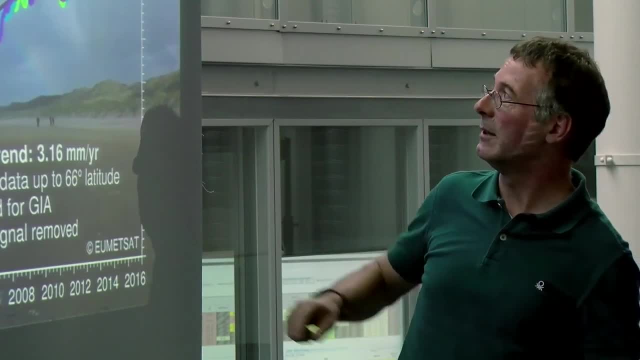 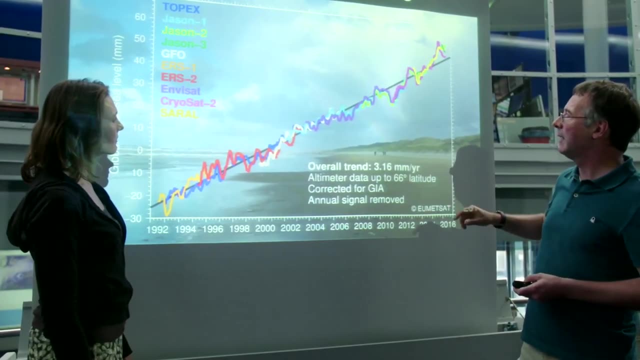 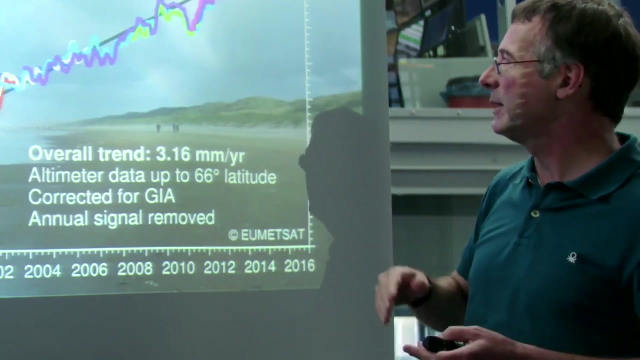 variations. we actually understand why that is. They are due to El Niños, For example. here we had a large La Niña and El Niño variation and you see that still in the mean And there is still a consistent trend of three millimetres per year. So every year it's about. 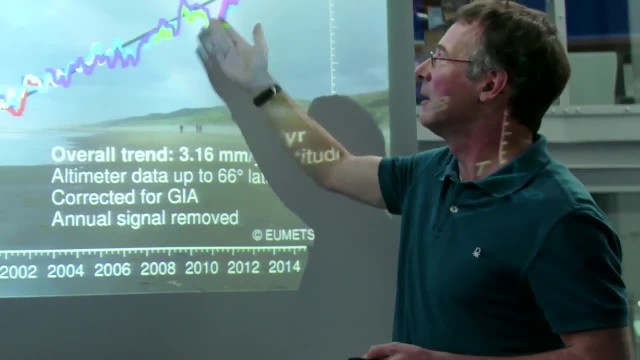 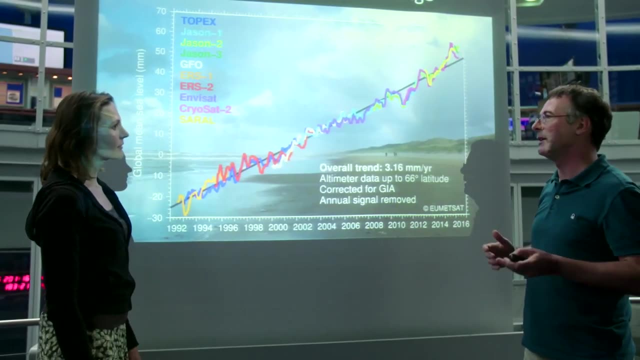 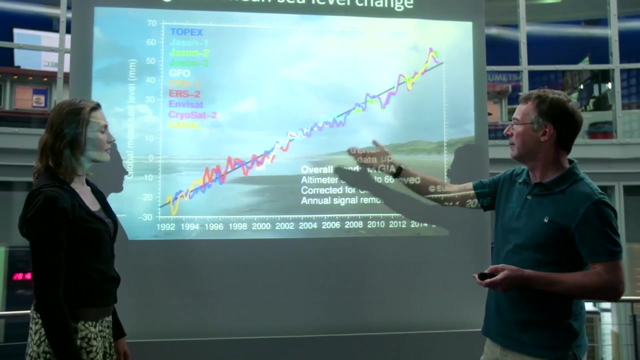 three millimetres. Some years are faster, some years are slower, but on average it is three millimetres. So don't focus on just one period, because there are variations and long-term variations. You can see sometimes as much as a decade long variations. but 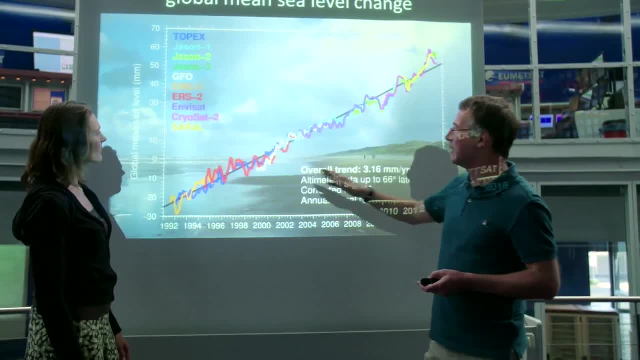 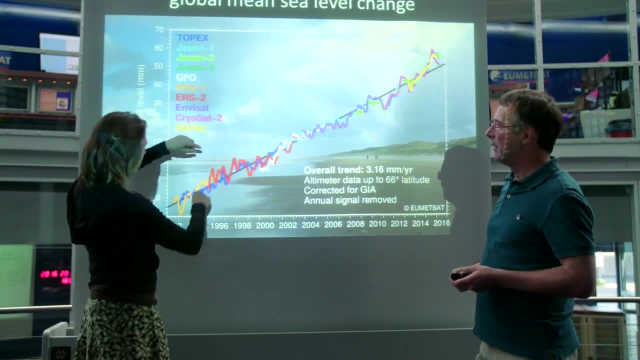 the trend is very clear And what is also very important is that all the altimeters basically are the same And these are all different. these are different satellites, so every colour on here- so the red one here- goes from there to there and then the yellow one kind of overlaps with- 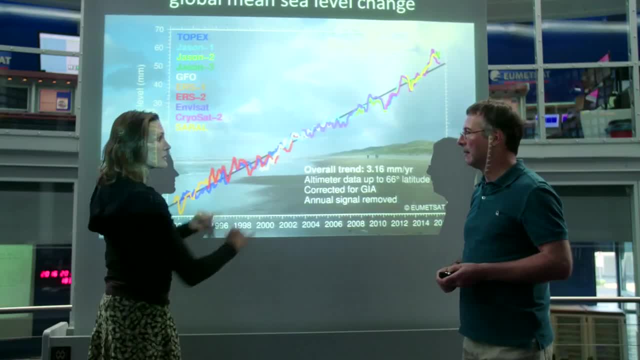 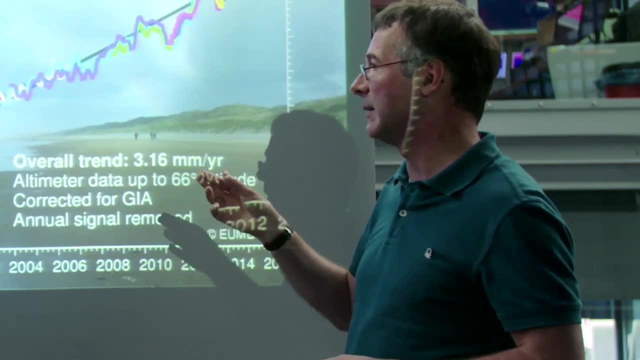 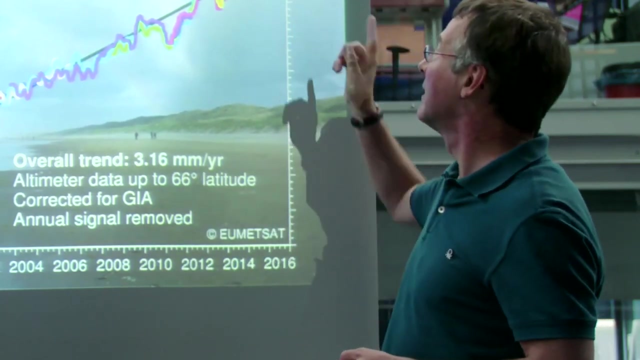 it, And so they're overlapping data sets from different altimeters. Yes, exactly, And that overlap is so important Because with the OpenLab, we can compare these satellites very well Now if they are running in the same orbit, meaning that they overfly the same track like Jason. 2. 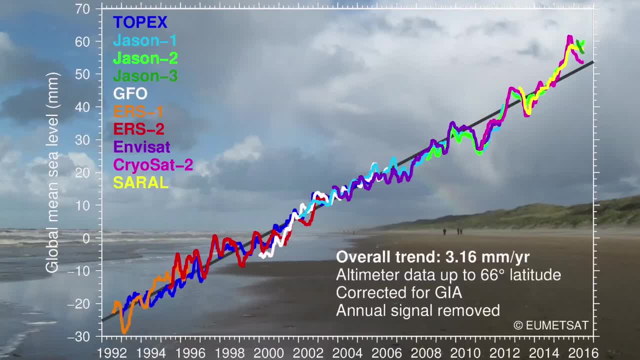 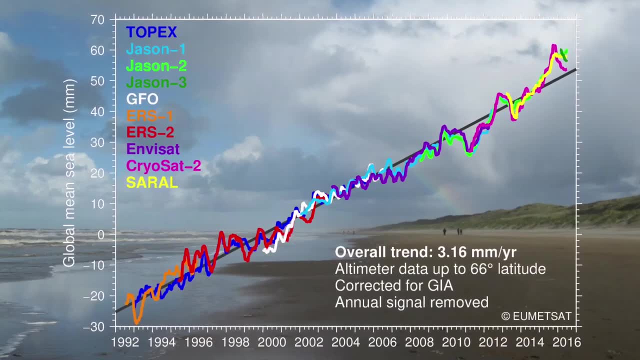 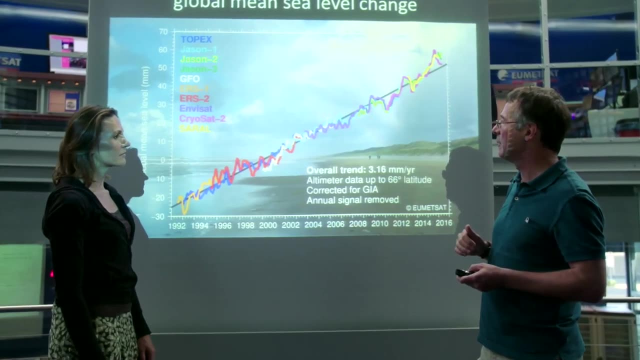 and Jason 3 are now. at this moment we can do that very accurately. In other cases it's not as easy, but still, because many missions, as you can see, have sometimes many years of OpenLab with others, we can do a very good job of aligning all these lines very well. 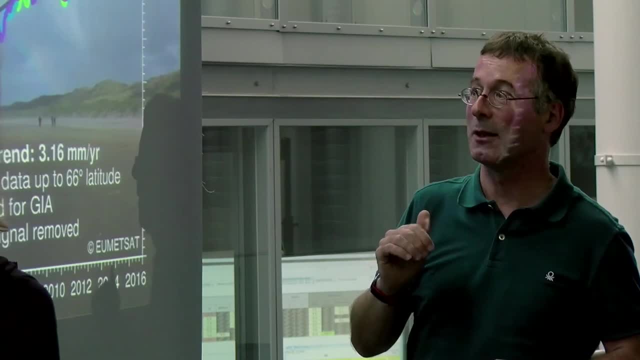 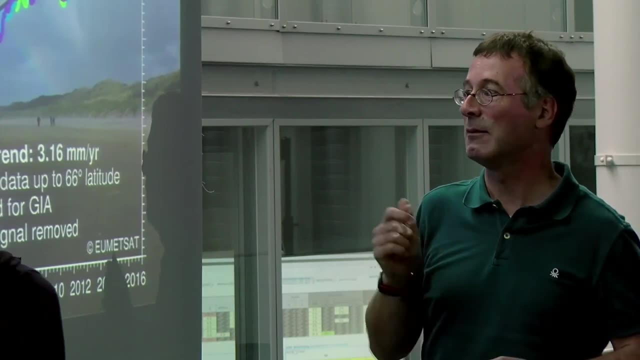 and understand, of course, when one is different from the other And of course, if you have three at the same time, as one is the outlier- we usually can figure out you know why was that? And sometimes it's instrumental. sometimes it's something that we did in the processing. 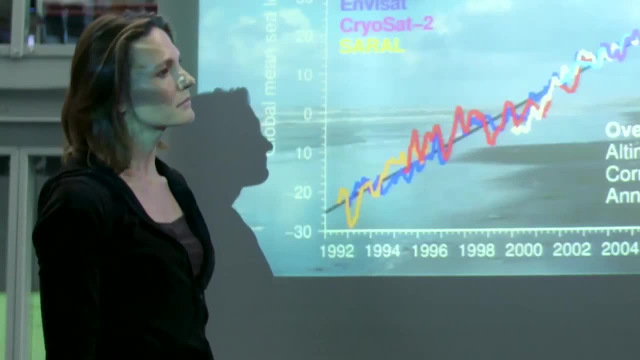 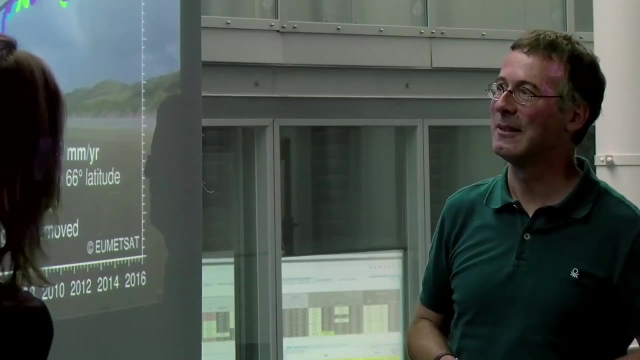 that was not done correctly. So we learn, and every mission learns from the other. But the overall picture is a sea level rise, and a very, very consistent one. So an eight centimetre change in the past 30 years doesn't sound like very much except. 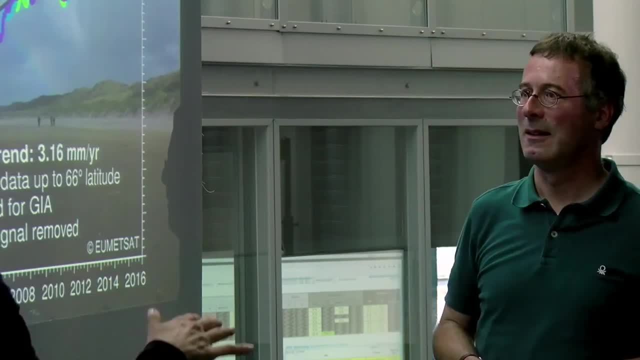 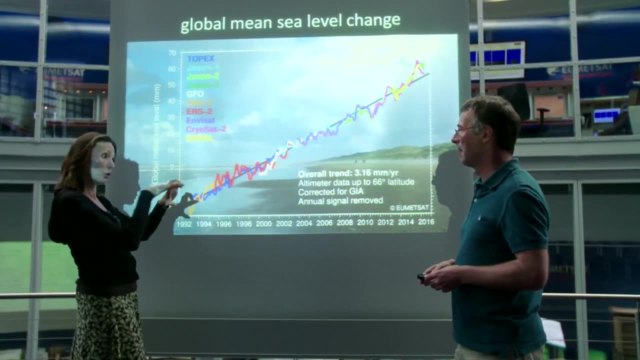 that our, Our infrastructure and the way that we, our harbours, are organised and the way that people on remote islands live. for them, that's a big difference, because if your tides come that much higher, they could go a lot further inland. 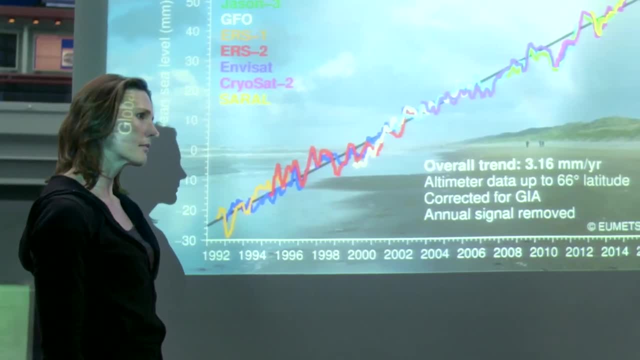 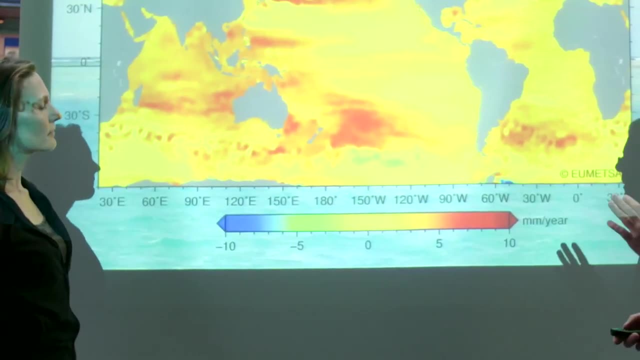 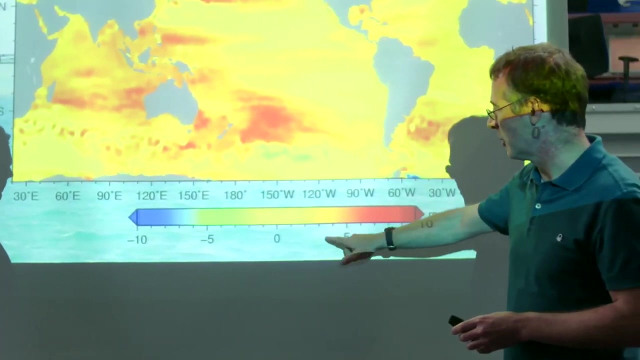 Yes, of course, And it's also not everywhere the same, And as you can see in this image. so here, over the same 25 years, you can see the local sea level rise. So we were saying that on average is about three millimetres. So then you're more or less in the middle. 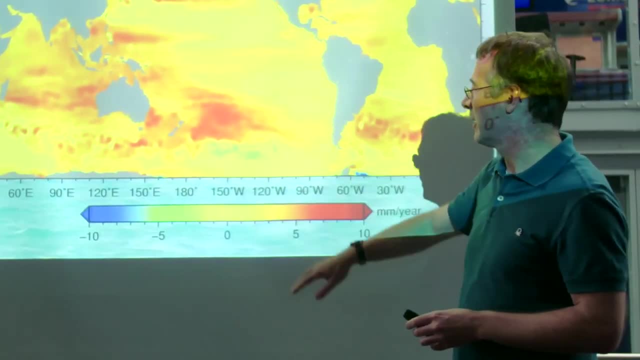 of the sea level rise than you are in the middle of the sea level rise, So you can see that the sea level is actually rising more. in areas in the Indian Ocean It's rising as much as five millimetres per year, But there are clearly areas where it's darker. 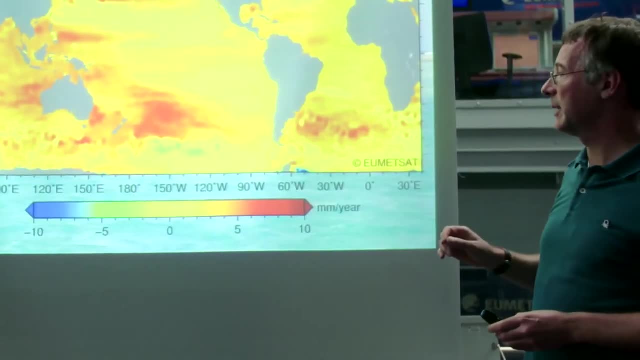 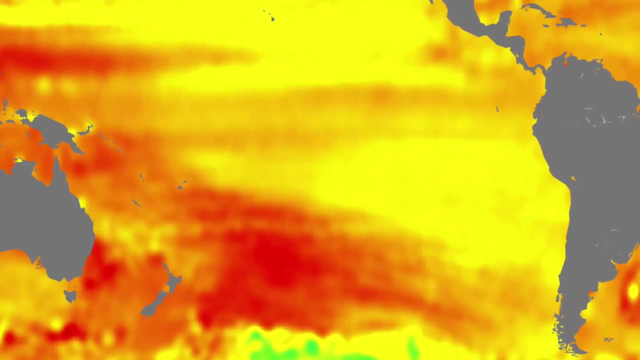 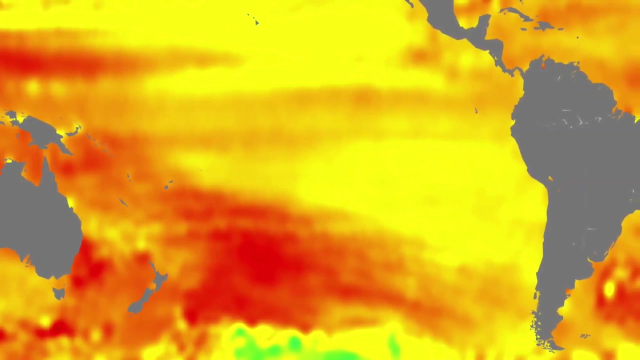 orange and red, and there the sea level is actually rising more. In areas in the Indian Ocean it's rising as much as five millimetres per year. Here in the South Pacific it goes even up to about a centimetre per year. So it's not homogeneous And actually we want. 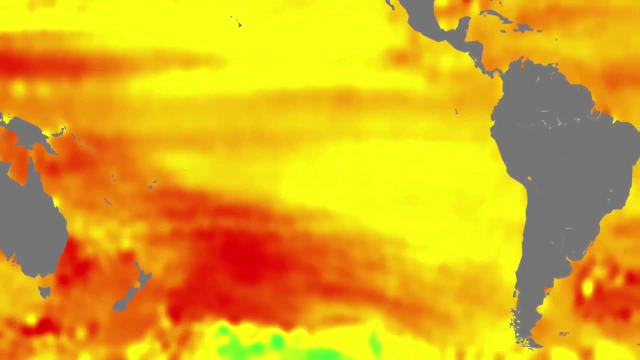 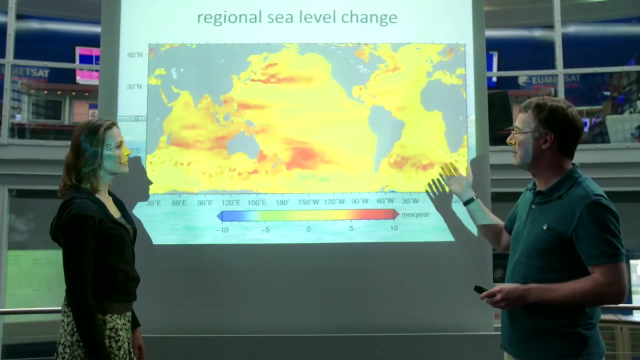 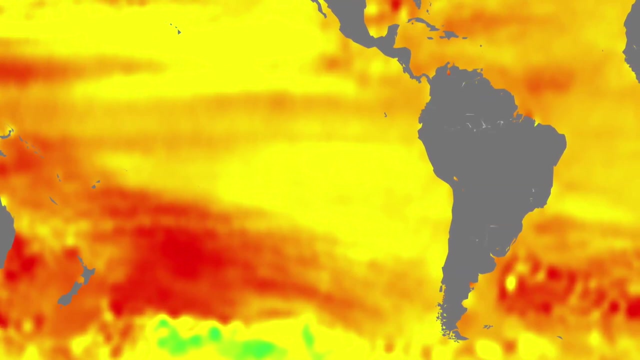 to learn why that is the case. Why is there? in some places it goes as more rise than the others. Of course, if you say melting of the ice, you would think that it will distribute homogeneously, which is in fact not exactly the case, because we're changing the gravity field as well. 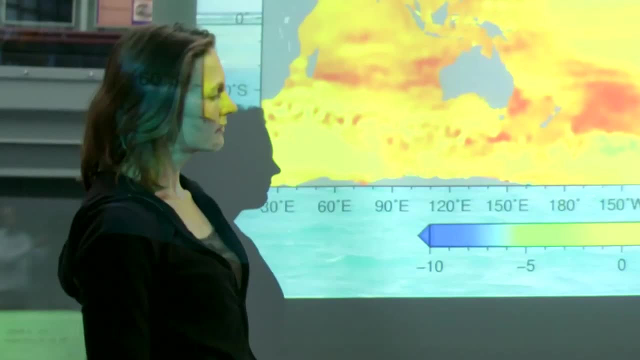 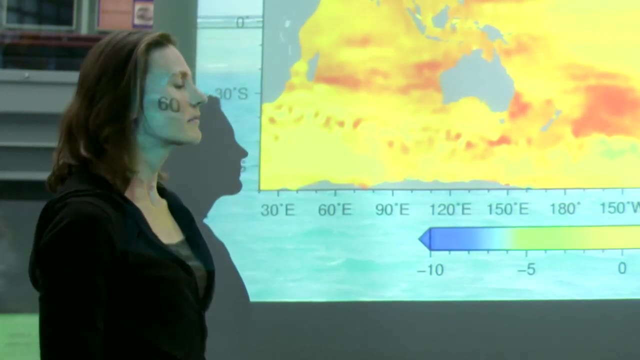 This is going a little bit far to explain that- But also, of course, because of the heating. in some places heating is more in other places And you see, there are variations that have something to do with the dynamics, And here we have a strong current, the Kuro-Shiro. 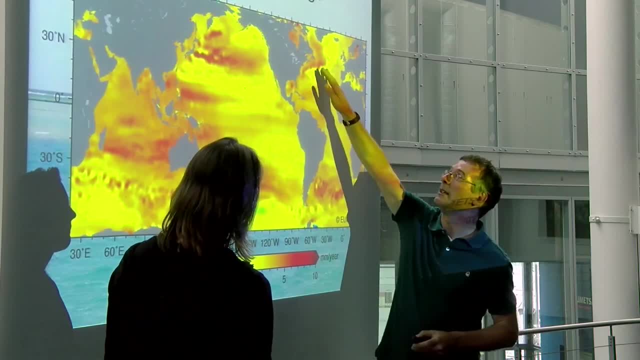 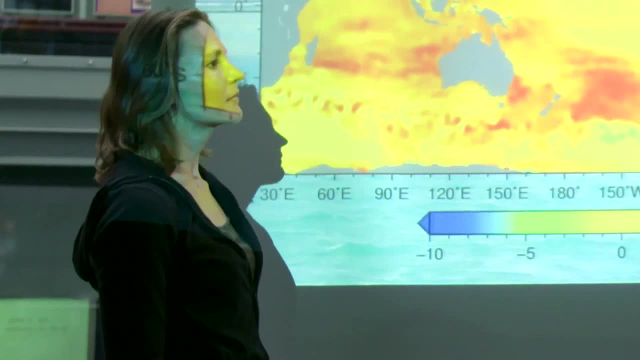 and here we have the Gulf Stream, And both in these cases we see a quite stark difference on either side of these currents. That can mean a lot. It can mean that on either side it's more heating than on the other side. It can also mean that the current is slightly changing in strength or in position. 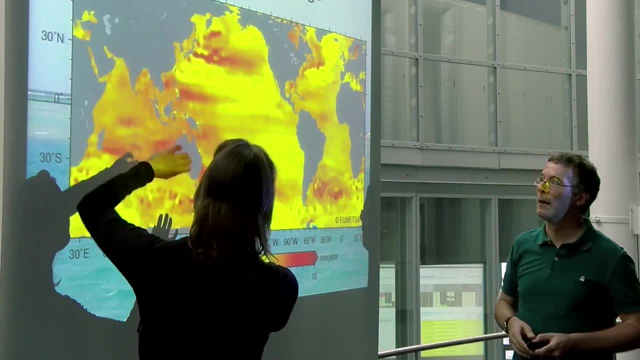 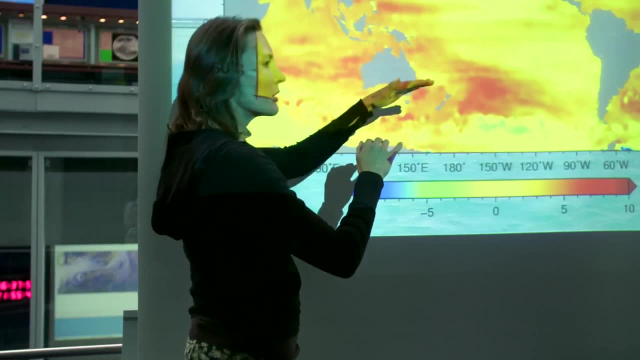 So this is very important data If you're living in one of these places, so you might have individual tide gauges, for example, around the coast. that said, you know it looks, maybe in this place, as though it's got a little bit higher in the past couple of decades. 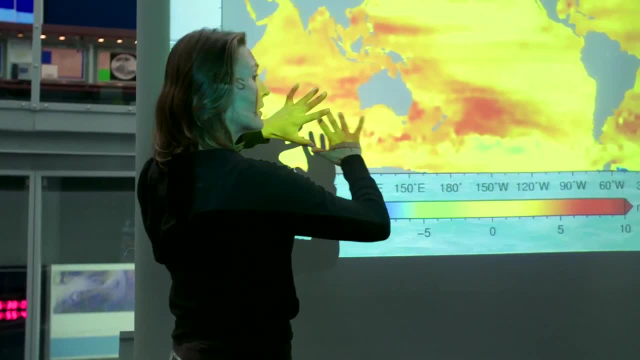 But this satellite data gives you this overview that shows you that the current is slightly higher in the past couple of decades. So you can see that the current is slightly higher in the past couple of decades. So this satellite data gives you this overview that shows you the big picture that sea level 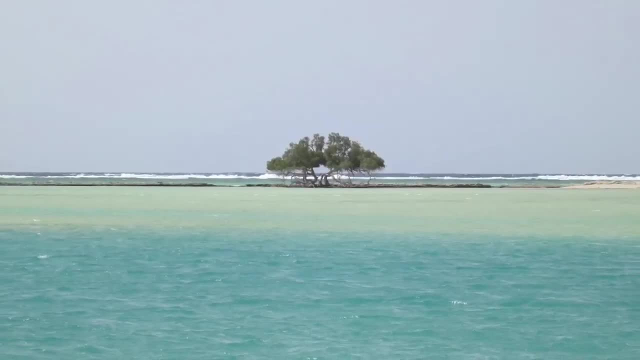 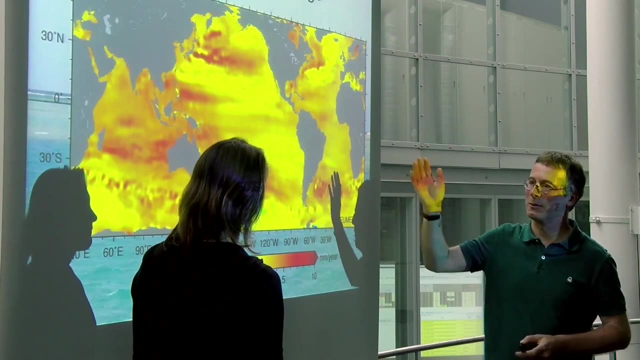 rise is going to hit some places a lot harder than others, And you can see where those places are. Yes, you can see that, And if you would plot in your tide gauges, you would, of course, find them mostly along the coasts, which, of course, is where it's most important. But 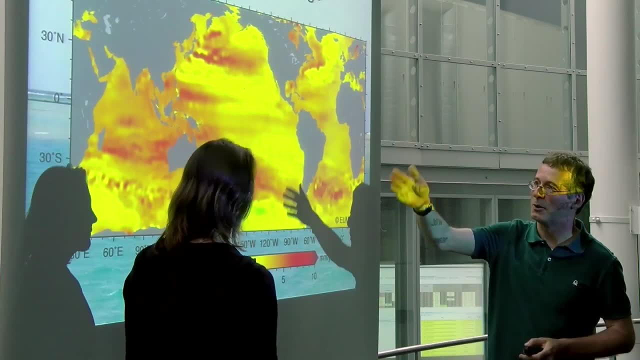 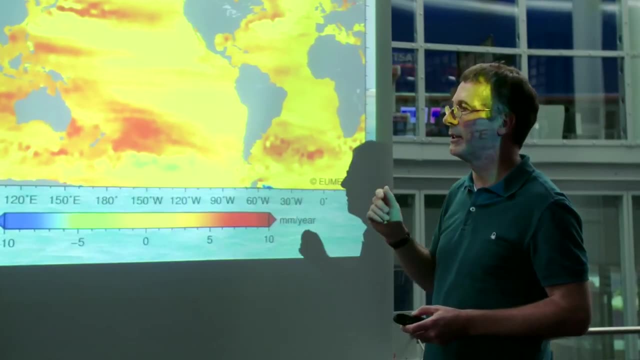 you would also find it mostly on the Northern Hemisphere and not in the Southern Hemisphere. So this indeed, gives you a global picture, this global picture of what is happening, and not just in the tide gauges. So this is a global picture of what is happening and not just in the tide gauges, Although, 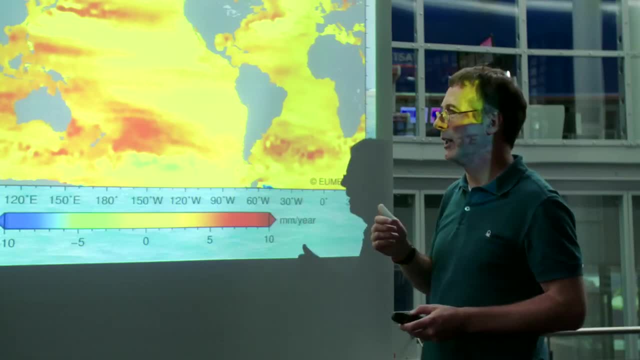 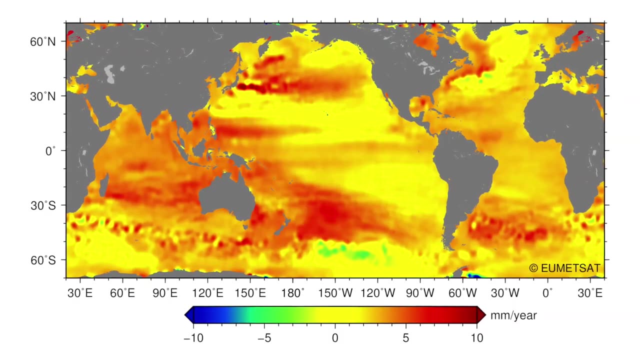 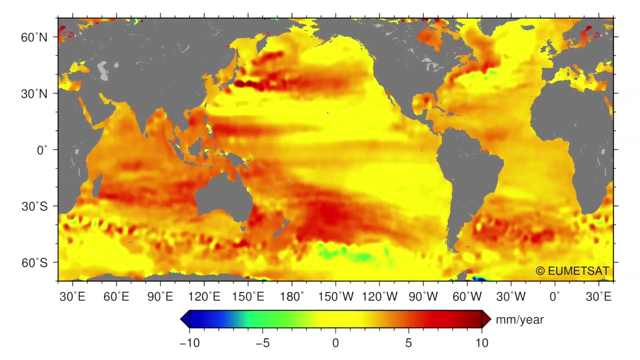 also, tide gauges can have a problem because you put them on land, And is that land stable? That could as well be changing itself, or the tide gauge might not have been properly embedded on rock, for example. Now, of course, it becomes a little bit more complicated when you start to say: you know. 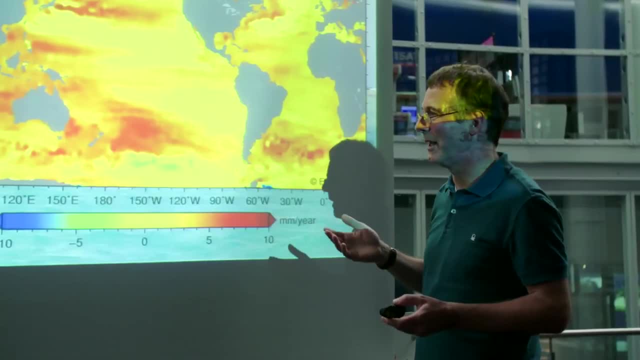 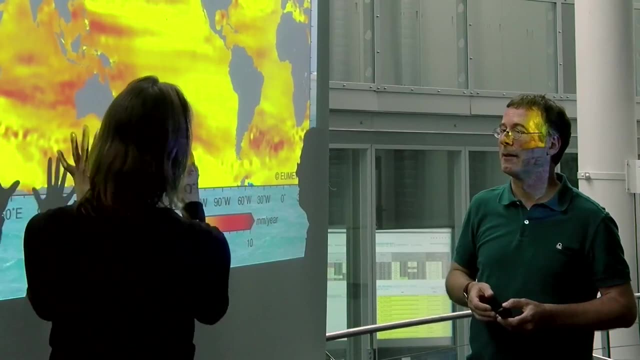 what is the sea level rise? Because, indeed, compared to the land, we need to think about it, And in some cases, it's worsened by the fact that land is at the same time sinking, And so this is the sort of information that is really useful to policymakers, for example. 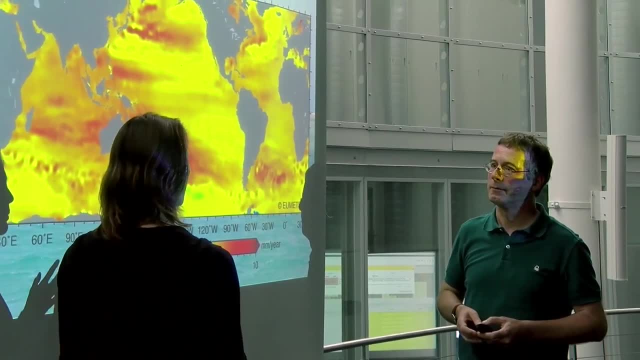 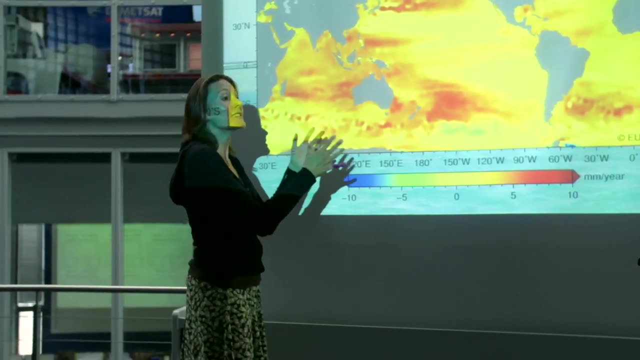 if a government is deciding whether to invest in flood defences or whether to try and protect a region from the sea or just to let it go. This is exactly the sort of data that is needed very practically by governments and local organisations to plan their future. 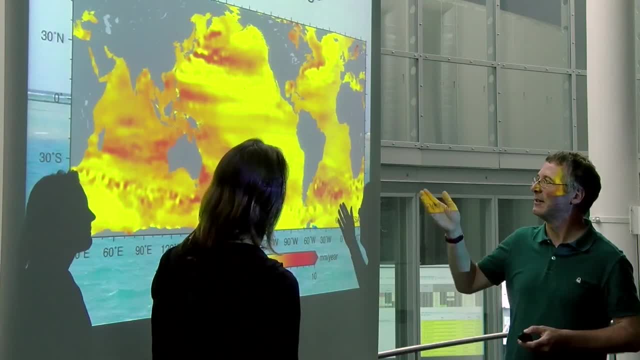 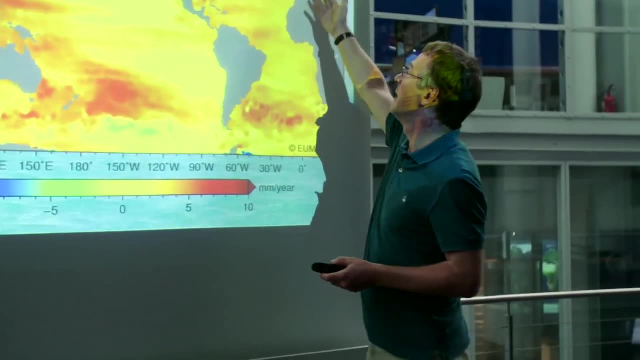 Yes, of course, because you cannot deny that these patterns are quite systematic. So if you look, for example, in the North Sea coast, we're actually not that far away, We're not that badly off. Still it is a positive number. So there is rise and we need to take care. 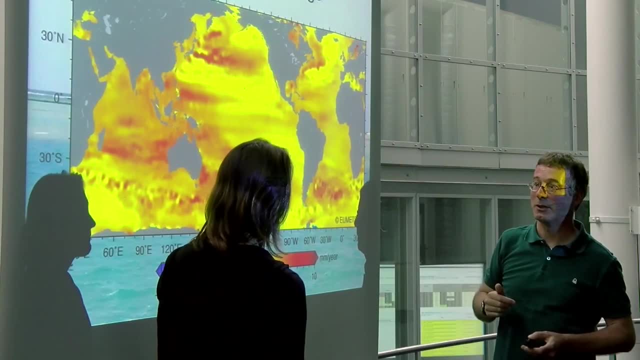 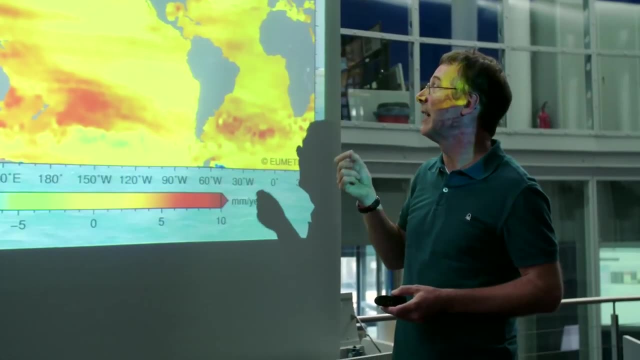 of it. Also in, of course, in the East Coast of the United States, where a lot of people living very close to the coast and exactly in that point where we need to consider that sea level is rising and you need to build up your defences because you have to raise. 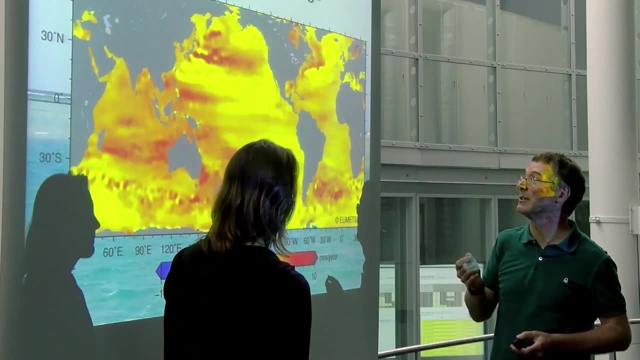 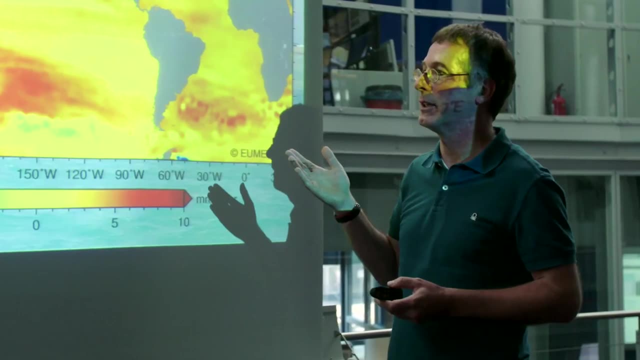 your dikes. you have to raise your levees, as they're called in the southern United States. You cannot just let it go as if nothing has happened. It is happening and it is very clear, And all these missions show the same thing.